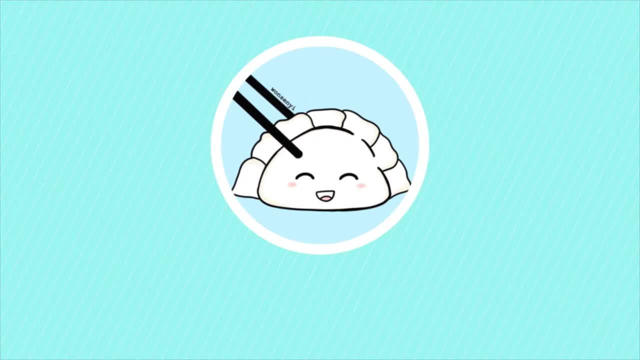 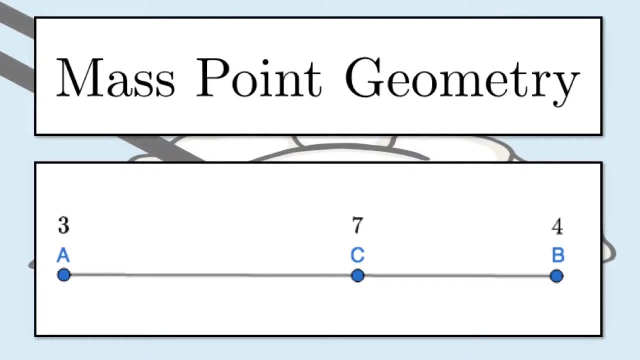 Hello everybody, it's Dumplet Jiaozai and welcome to the very first ever Dumplet Tutorials. Today's topic is on Mass Point Geometry. From the name itself, it's used in geometry And this is a very, very nice technique shortcut, or whatever you want to call it. 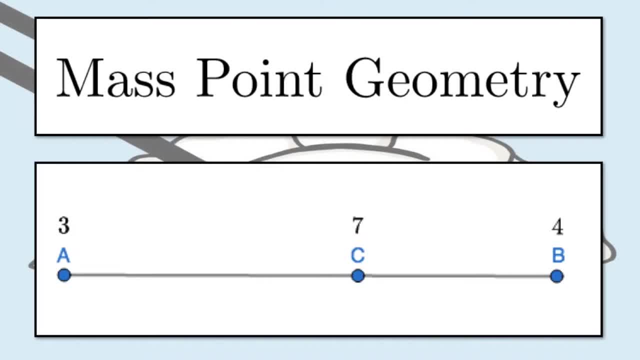 In a lot of the geometry items. it's seen in mathematical proofs. it's also seen in short answer problems. Well, it's a very, very common technique to use in Olympias as well. So, without further ado, let us dive into today's topic. 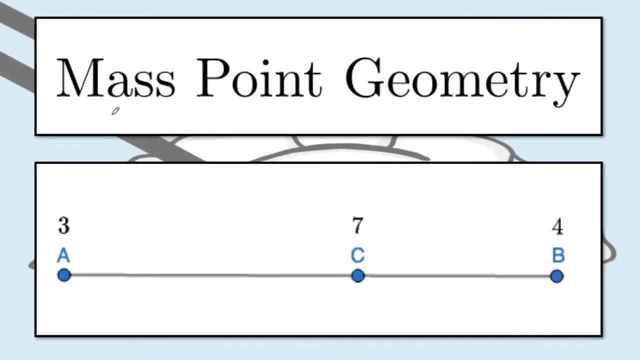 Now the concept of Mass Point Geometry is very simple. You have masses on a point, on a geometric figure. Now let's have this figure below: We have segment AB with point C. on segment AB, The 3,, the 7, and the 4 here are called weights. 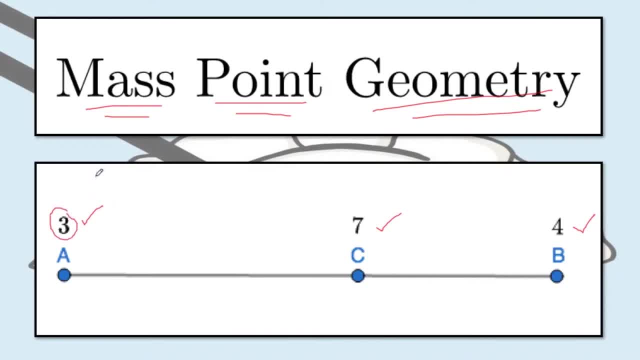 So we say that 3 is the weight or mass assigned to point A, 7 is the weight or the mass assigned to point C and 4 is the weight or the mass assigned to point B. And this is an example of a balanced figure. and we say that this is the distribution that keeps segment AB balanced. 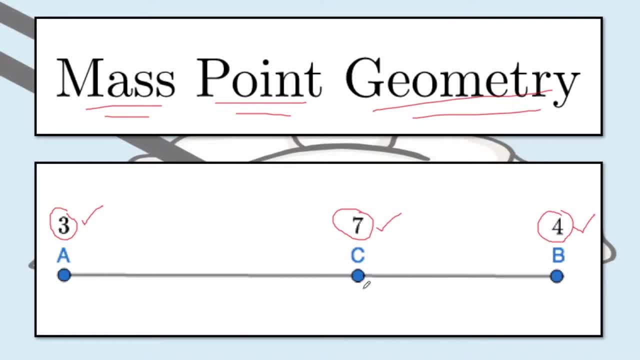 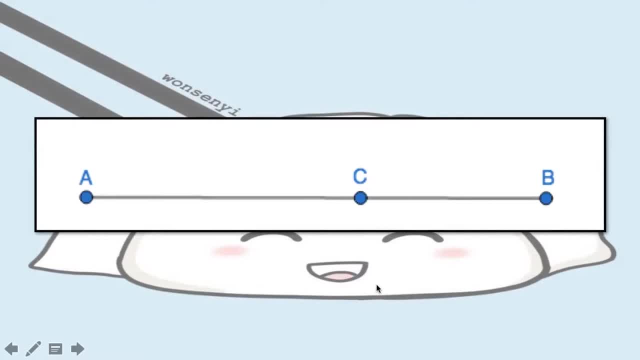 Now let us try to go into why this is balanced. Now, the concept of Mass Point Geometry comes from physics, but we're not going to talk about physics here. Let us make things simple. The concept is that: suppose you put your finger on a stick. 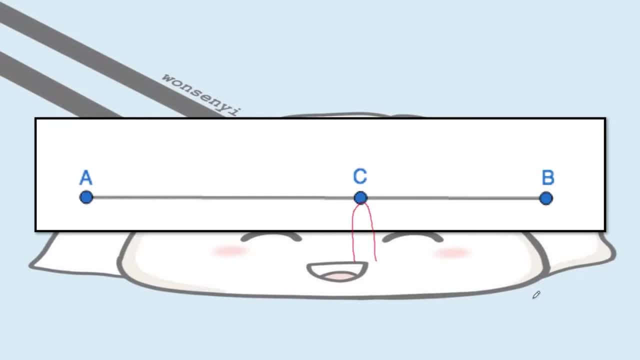 Let's say the stick is segment AB. If I do nothing and I just literally put my finger on point C, on the center, what's going to happen? Well, point A will tend to go down and point B will tend to go up. 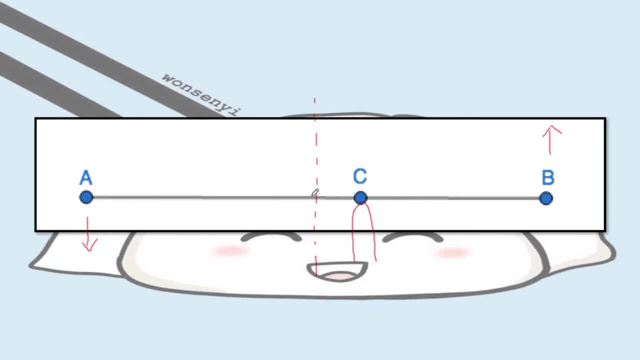 Because AC is longer than CB. So AC is longer, which means it's heavier. So point A tends to go down and point B tends to go up. Now, if my finger was in the middle instead, then it's going to be balanced. 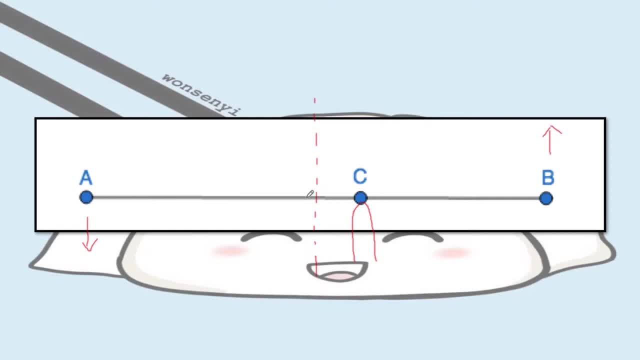 Since you know it's in the middle, it's also called the center of mass for the physics people out there. So that's the concept behind Now. why do we assign weights or masses? Because this is a segment and it doesn't move. obviously. 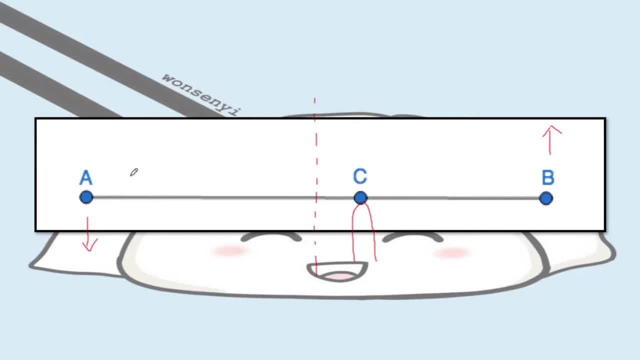 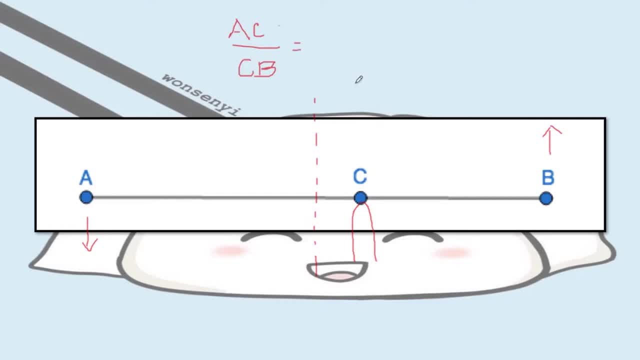 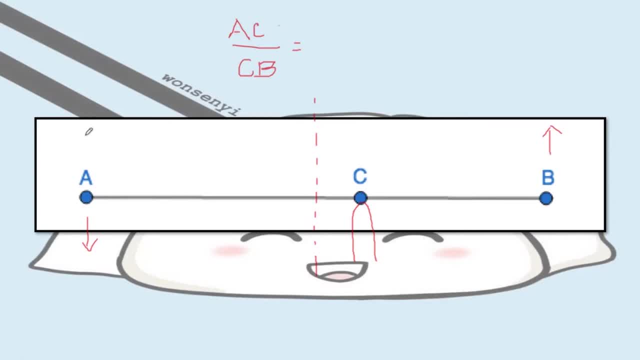 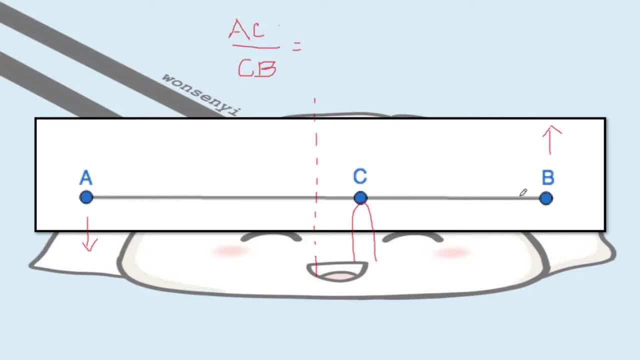 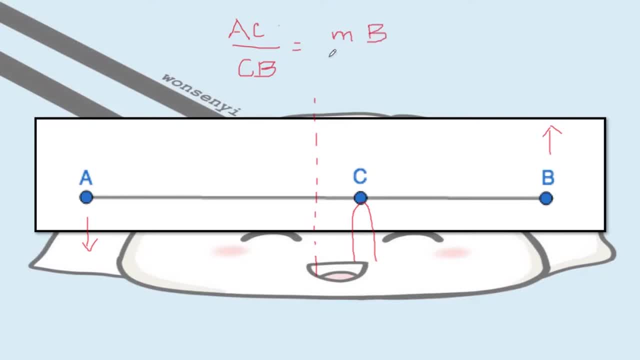 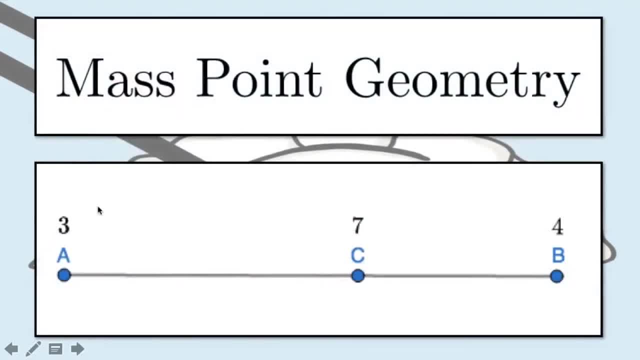 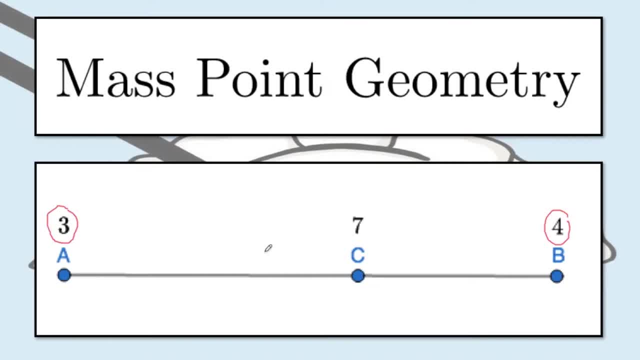 assigned to A, which is true. So since the weight assigned to B is 4 and the weight assigned to A is 3, then we can conclude that the ratio AC over CB, so the longer segment to the shorter segment, equals the larger weight obviously, to the smaller weight assigned, 4 and 3.. Now what is? 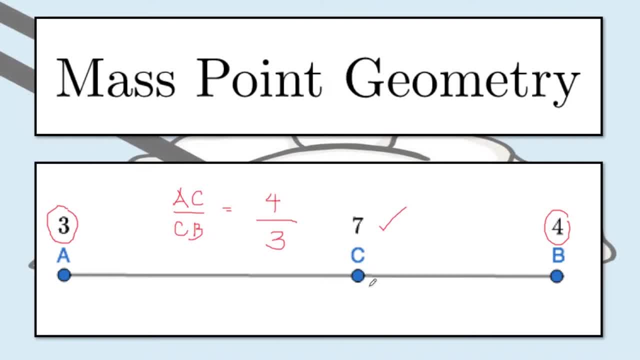 the 7?. 7 is actually the total mass on point C. Why? Because 7 is 3 plus 4.. Now if you put 3 on A and 4 on B, then obviously the total mass on C would be 7.. So this is the concept of mass point. 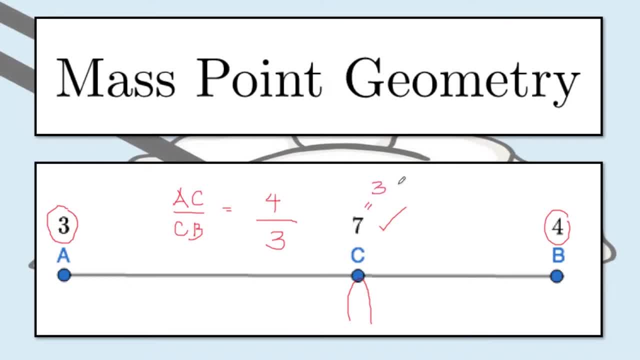 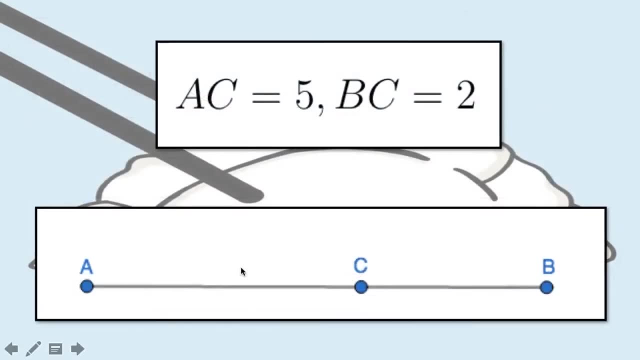 geometry. So we have the 7 here that came from 3 plus 4.. Now this is the very, very basic concept of mass point geometry. Now let us dive into some examples. Suppose I have AC equals 5 and BC equals 2, and I want to make this figure balanced. 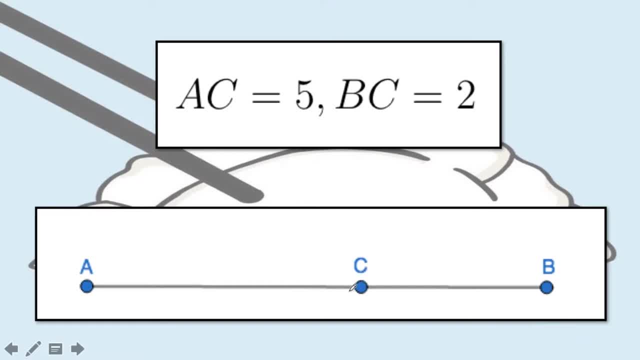 All right. So first step, I must assign weights to points A and B. So since AC is longer than CB, I already know that I should assign a heavier weight on point B and a lighter weight on point A. So I must have the ratio: 5 is to 2, which is AC over CB or BC. 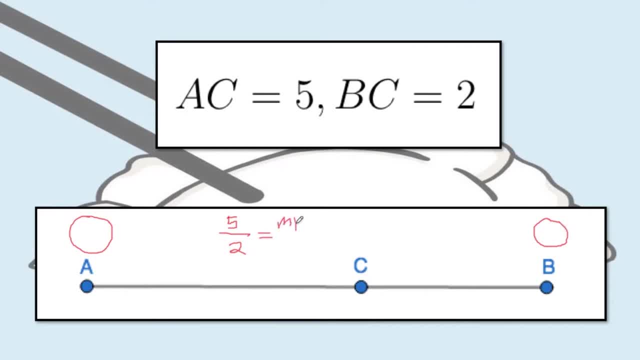 This is equal to the mass on B over the mass on A. Now, very simple. I can easily assign the weights 5 and 2.. But note that these are not the only answers. Obviously, any combination of masses that have the ratio 5 is to 2 is going to work. So I can, instead of 5 and 2, I can put like 10 and 4.. 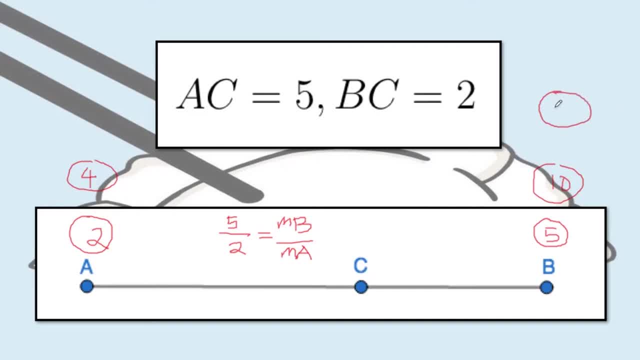 If I want to go even more bizarre, I can go 1.5 and 0.6.. So there's a lot of masses that you can assign. Just make sure that the ratio is going to be preserved. So like AC over CB, since that's 5 is to 2, then the mass on B to the 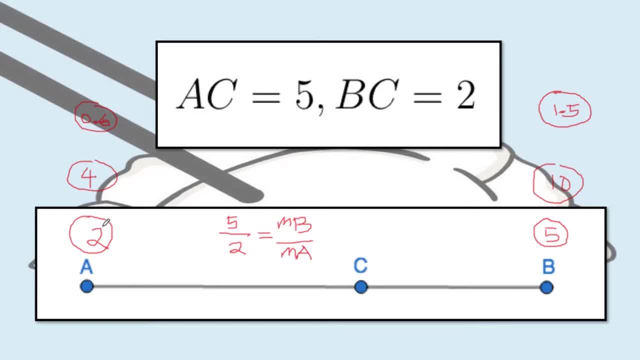 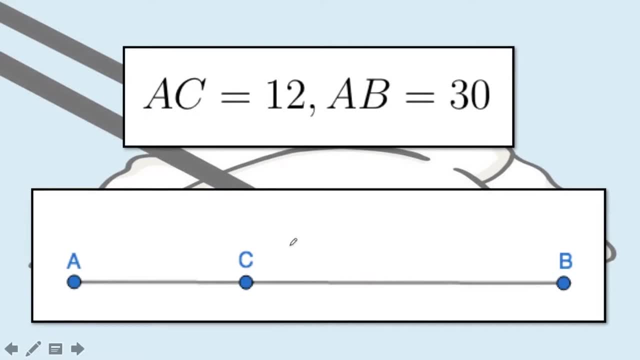 mass of A. the ratio should also be: 5 is to 2.. As another example, let's say AC equals 20 and AB equals 30. So a very common trick. Note that AB is the entire thing, So AB equals 30. From that, 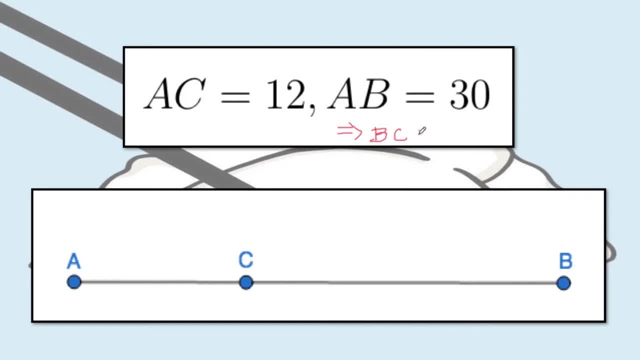 we can deduce that BC equals 18.. So the ratio is actually 12 is to 18.. So AC is shorter than BC. So 12 is to 18, which is also equal to 2 is to 3, because 12 over 18 is. 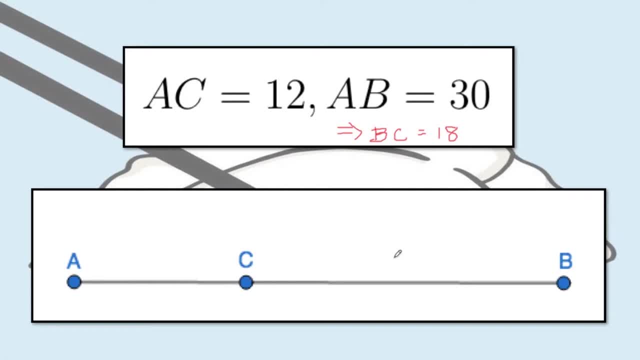 indeed 2 thirds. So in fact I can use the weight 2 and 3.. So 2 will be assigned to point B because BC is longer than AC. So the smaller weight is assigned And I'll assign a point. I'll assign. 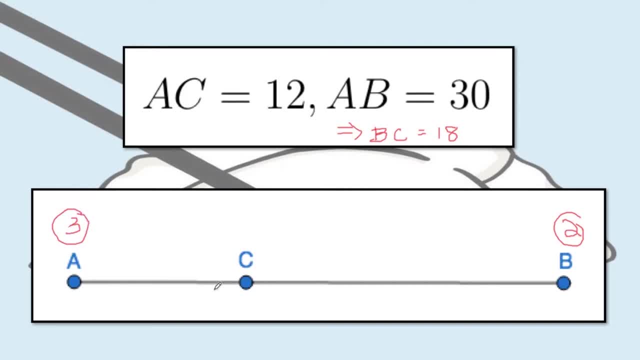 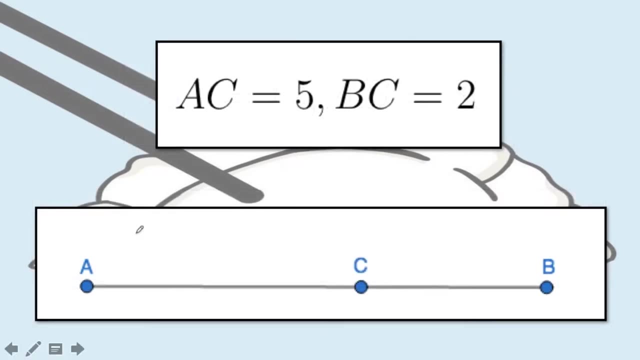 a mass of 3 to point A, since AC is the shorter. Now, on point C, we can assign. we know that the weight would be just simply the sum of these two. Now in a previous example I forgot to mention, since I can assign a weight of 2 here and assign a weight of 5 here. on point B: 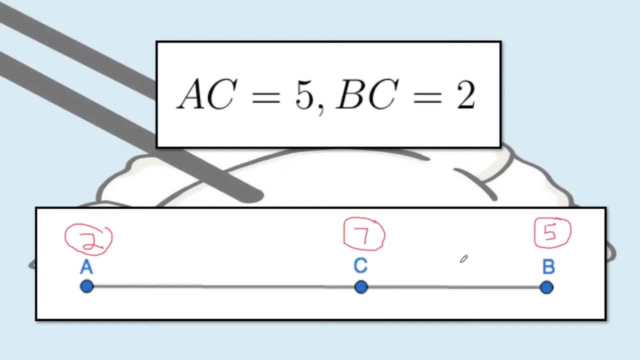 then the weight on C would be 7.. So simply add them. Now, obviously, if I use 10 and 4,, then the weight in the middle should be equal to 14.. So we must be consistent. Whatever numbers we use, obviously those are the numbers that we're going to add. If I used some bizarre. 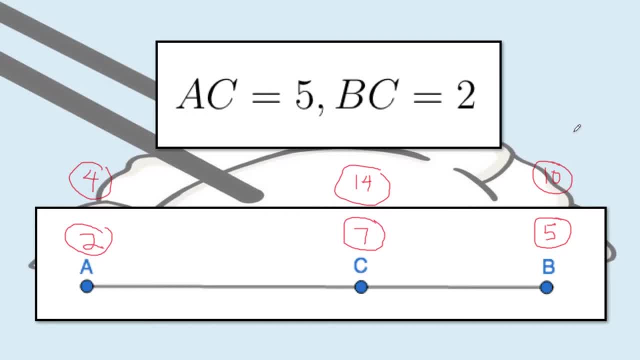 numbers like 0.6 and 1.5, as seen in the example a while ago. then I would add 0.5 and 1 plus 6 to get the value or the weight on C. So applying these two concepts, let us go to the most used. 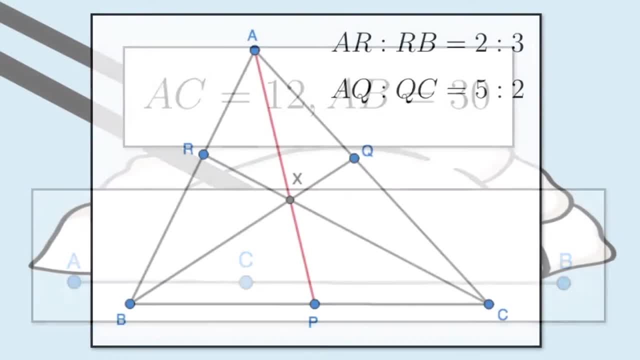 figure in a lot of the geometric items, the triangle. Now, here there's a lot of segments And we can use mass points geometry to balance each and every one of them, And that's going to help us, since we know that we can convert ratios to masses and we can convert masses. 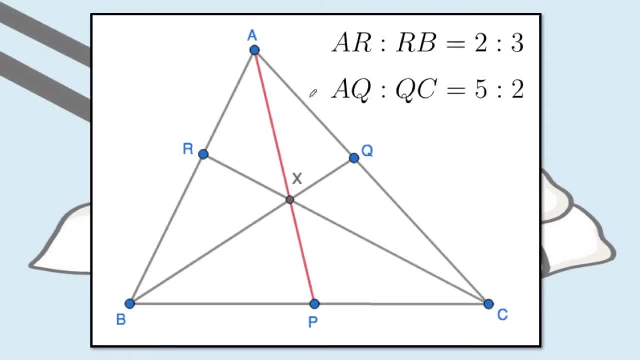 to ratios as well. So let us start with this item. AR is to RB is 2 is to 3.. By the way, this figure is not drawn to scale. So AR is to RB is 2 is to 3.. So AR is shorter than RB. So let's focus on segment AB first. 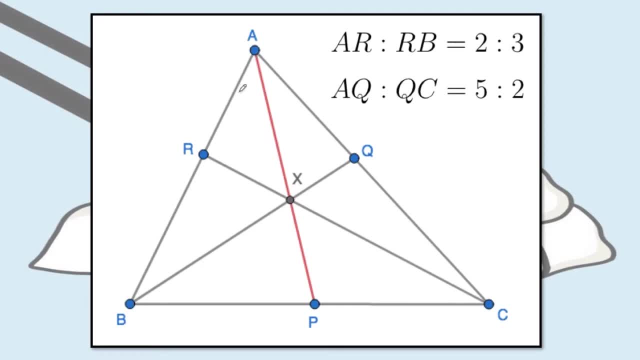 Let's say we want to balance segment AB. Since AR is shorter than RB, the weight on A should be greater than the weight on B. Now the ratio should be of the form should be: 2 is to 3.. So the heavier weight on A I can easily use the weight 3 on A, then I'll assign 2 on B. 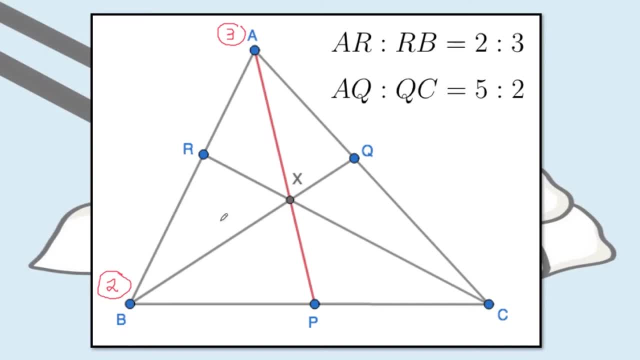 Now the ratio is indeed preserved: AR is to RB is 2 is to 3, which is the ratio of the mass in B over the mass in A. Now let's focus on AQ is to QC is 5 is to 2.. So AQ is: 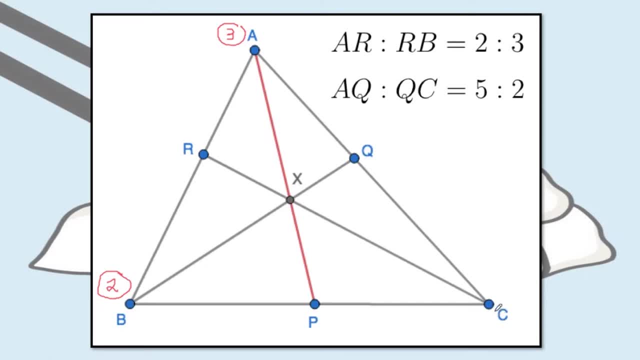 the QC is 5 is to 2.. Again, the figure is not drawn to scale, But on the ratio. we know that QC is shorter than AQ. So the weight on C to the weight on A is 5 is to 2, so we. 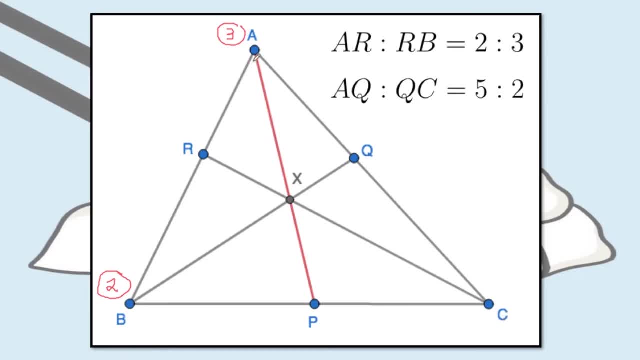 can exchange both on B to QC and the other way around. So I willHis mue Suk: 15 points points to 2.. So that's thekuelsma2 in R1. should be of the ratio: 5 is to 2.. 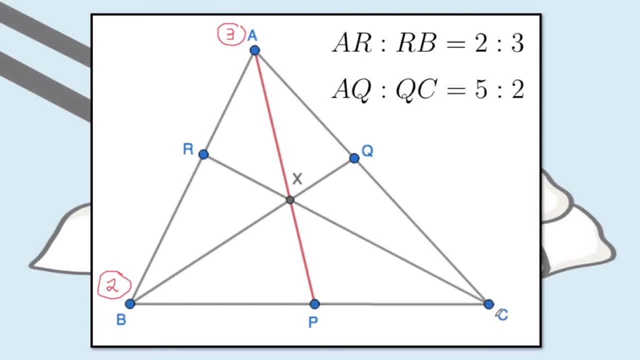 Since QC is shorter, the heavier weight should be assigned to point C. Now there's already a weight of 3 on point A, So whatever we put on point C, it must be in a 5 to 2 ratio, when dealing with the mass of C, to the ratio of the mass of A. 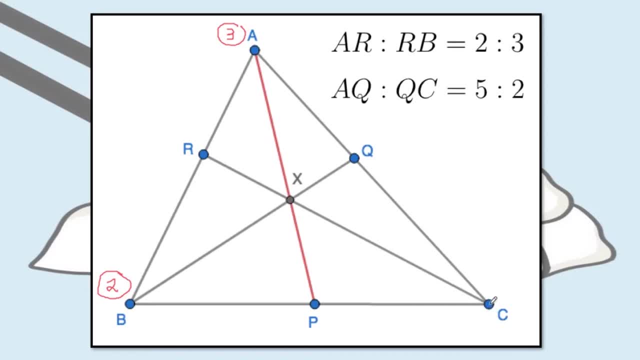 Okay, so the weight on C over 3,, so the mass on C over 3, this should be equal to 5- is to 2.. So the weight here should be 5.. 5 halves times 3, so the mass on C would be 15 over 2.. 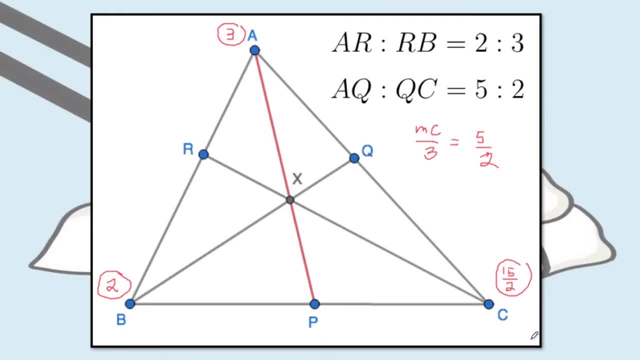 Now note how segments AB and AC are done. so we can easily get the mass of R and Q. So let's get R first. so it's just 2 plus 3, since 3 is assigned to A and 2 is assigned to B. 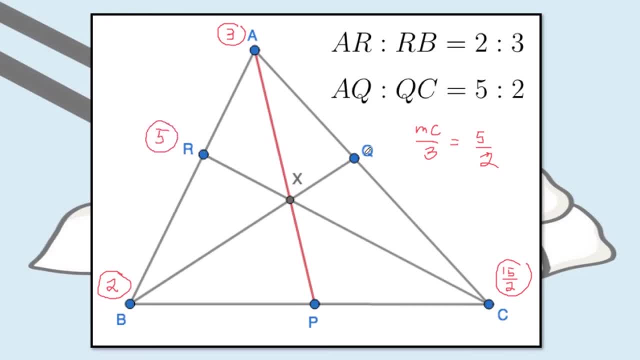 So R here would have a mass of 5, and Q here would be 3 plus 15 over 2,, which gives us 21 over 2.. Now segment BC: here is already balanced, since we have masses on B and C. 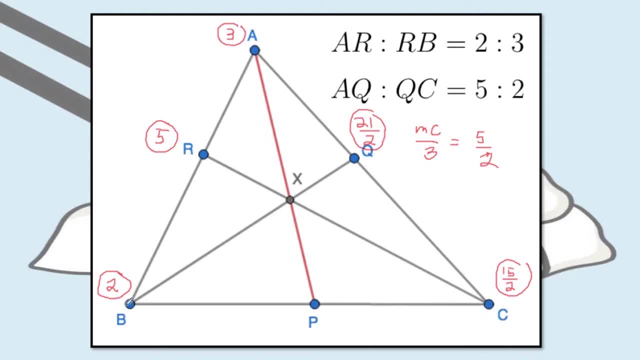 So 2 plus 15 over 2 would give us the weight on P. So 2 plus 15 over 2, that's 19 over 2.. So 19 over 2 is the weight on point P. 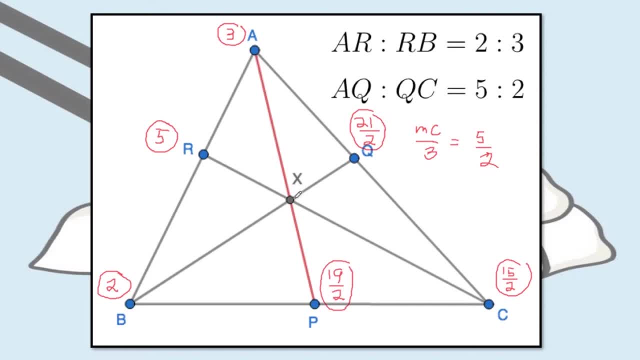 Now, lastly, we can get X in a lot of ways. We can use segment BQ, segment RC or segment AP. Now let's just use segment AP, since it's already highlighted. So segment AP. so 3 is assigned to A. 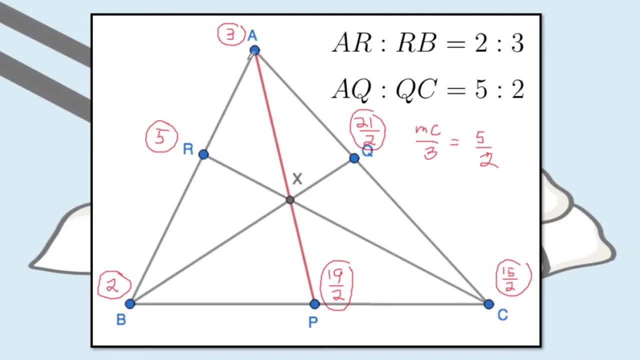 19 over 2 is assigned to P, So the weight on X should be 3 plus 19 over 2, and that gives us 25 over 2.. So the weight on X is 25 over 2.. Now, whatever segment you use, 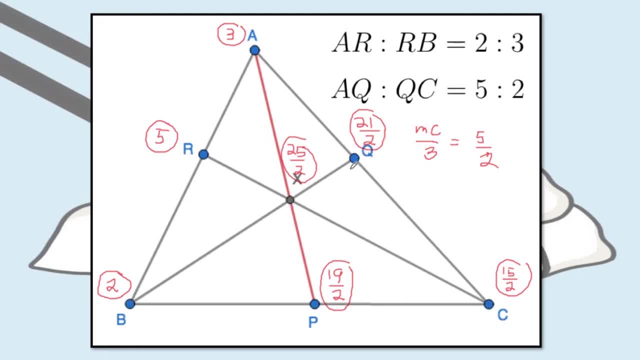 note how you're going to get 25 over 2.. Let's consider segment BQ: The weight on B, which is 2, plus the weight on Q, which is 21 over 2, if you add them it's going to become 25 over 2.. 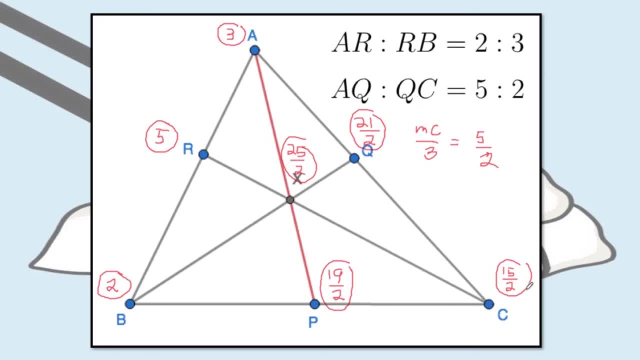 Same can be said if you use segment R or segment RC. 5 plus 15 over 2 is equal to 25 over 2.. So since all the ratios are correct and all the sum-takens are also correct, we can conclude that we have finally put this triangle in equilibrium. 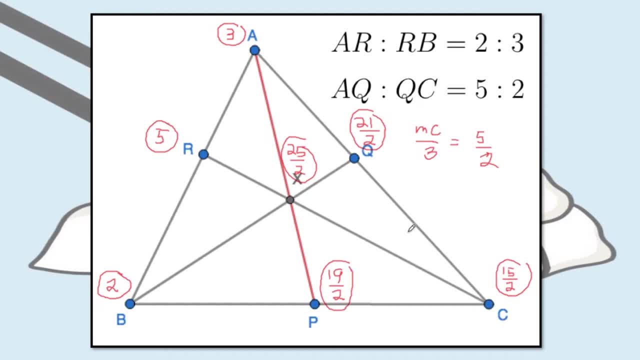 So we have successfully made the correct distribution of weights and we are able to get all the other ratios that this triangle has. So, aside from the AR equals, RB is 2 is to 3, and the AQC is 5 is to 2,. 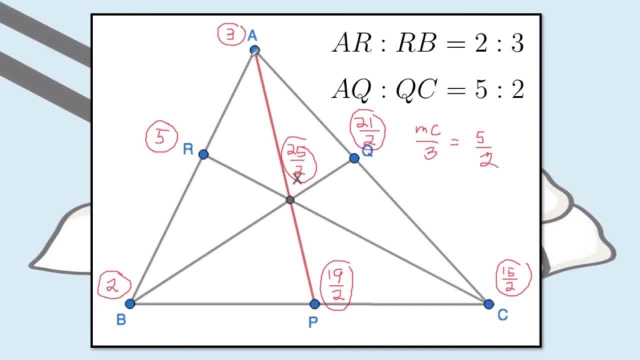 we can get a lot of information. So let's just say, on segment AP- Oh, this is point X, just in case you don't see the X. So on segment AP, we can get the ratio AX is to XP. 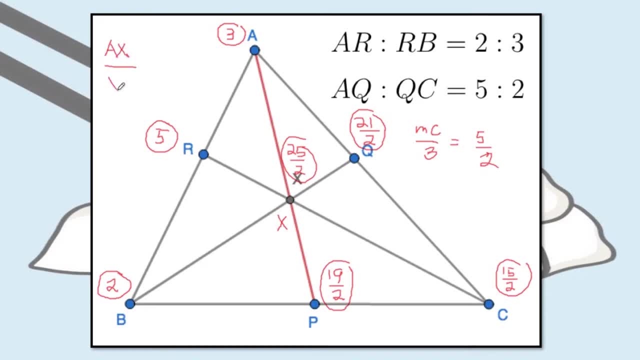 Why? Because we already have the weights on A and P. So let's try to get AX over XP. Now. AX over XP. the ratio of that should be equal to the weight on P over the weight on A. So it's like AX is to XP equals 19 over 2 over 3.. 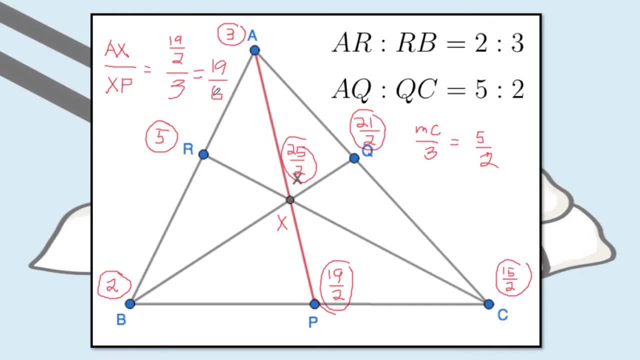 And this would give us 19 over 6.. So that's just one of the ways you can get it And for fun, you might want to get on. what are the ratios of BQ? sorry, of BX is to XQ and RX is to XC. 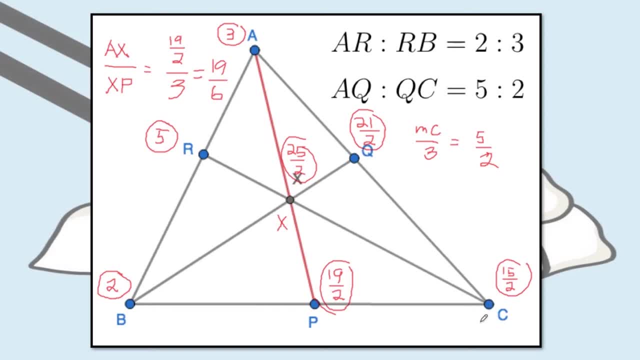 Now, you can do it. You can try to do it and leave your answers in the comment section below. Now for an exercise. let's have this item. So same thing. I've given you two sets of givens and try to put weights on this triangle such that it is balanced. 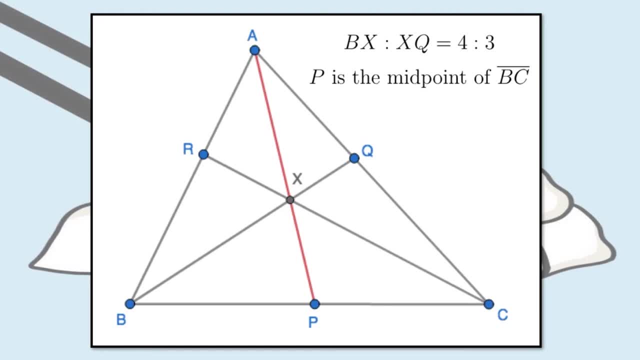 Now again, you can pause this video, give yourself some time to complete the triangle, to put weights on the triangle, all right. But if you're done, let us go assign the weights, All right. So the first ratio is a ratio, just like the previous example. 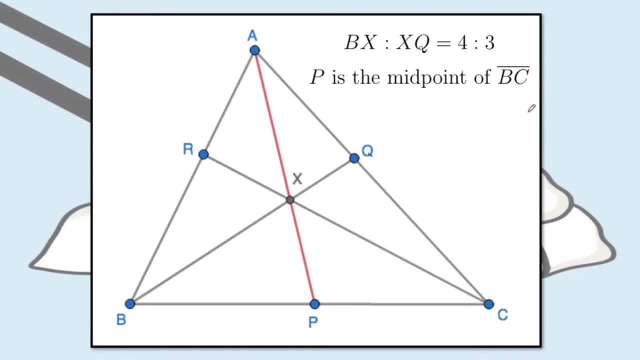 Now the second thing. the second given P is the midpoint of segment BC. This is just another fancy way of saying BP equals PC, since P is the midpoint. So from here I can get BP. So BP is to PC is 1 is to 1, since they're indeed equal. 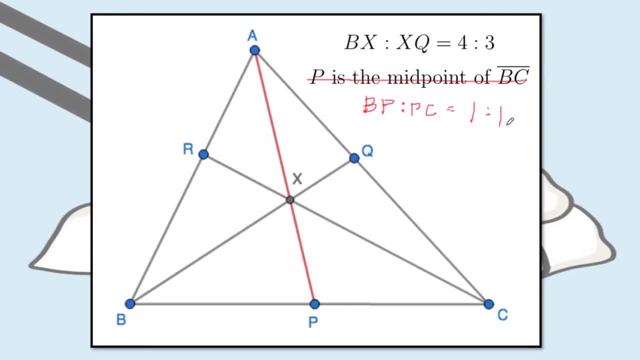 Now everything would be the same, just in the previous example. Now you can start with literally any segment you want. Well, obviously you must start with, you know, one of the given segments. So BX is to XQ or BP is to PC. 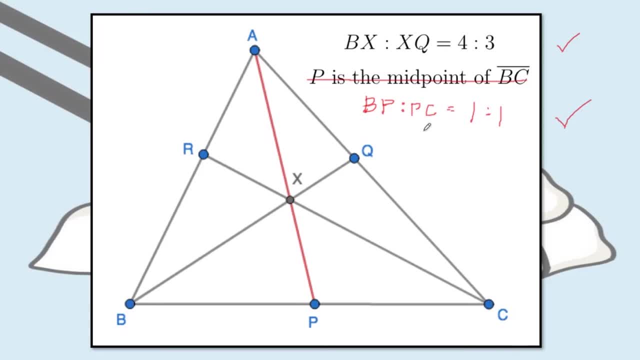 So let's start with: BX is to XQ. Now, if you started with BP, BP is to PC. don't worry, you will be getting the same answer. It may be not the exact same of value, the exact same set of values, because 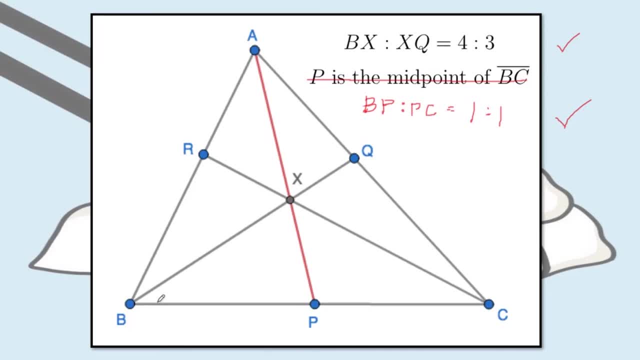 as I mentioned, you don't, as I've mentioned, like if you have, BX is to BX is to XQ, is 4 is to 3, you don't really have to assign 4 and 3.. You can use 8 and 6,, 12 and 9 or any other numbers. 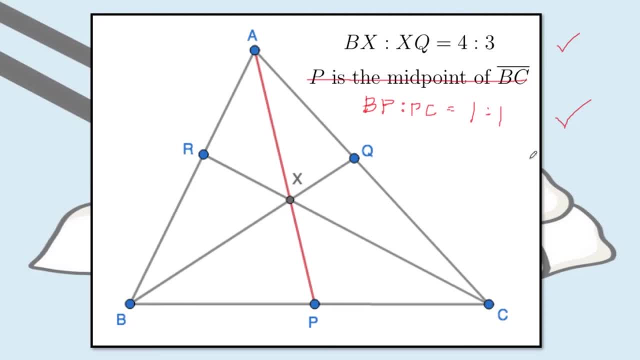 number combinations that have the ratio 4 is to 3.. So if you want to check your work, just check all the sides and all the ratios to check if it's correct. And if it is, if it's satisfied, then your, then your. 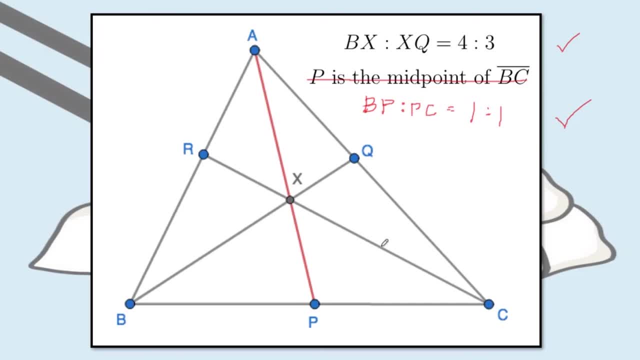 then your weight assignment is correct and your triangle is balanced. Now let's just go go through this. So BX is to XQ, is 4 is to 3. So BX is longer than XQ. So conveniently I can assign 4 to Q and then 3 to B. 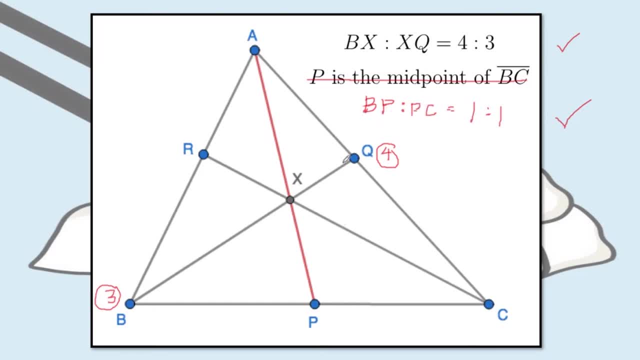 Next let's talk about BP is to B, BP is to PC is 1 is to 1.. It's convenient since I already have the 3 on B, So I know point C should also have a weight of 3, since 3 is to 3 is 1 is to 1.. 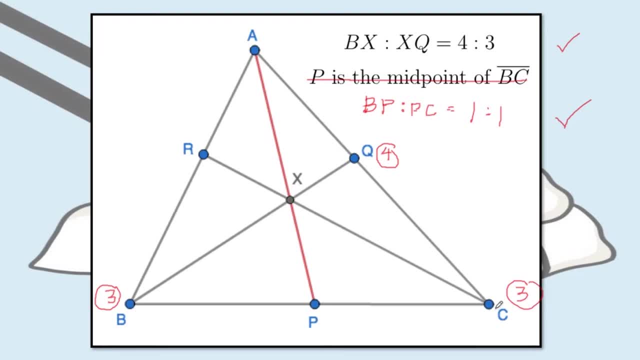 Now I can get the weight on P because I already have B and C, So 3 plus 3, that gives me 6.. Oh, on X as well, I can get the weight on X, since I already have segment BQ. 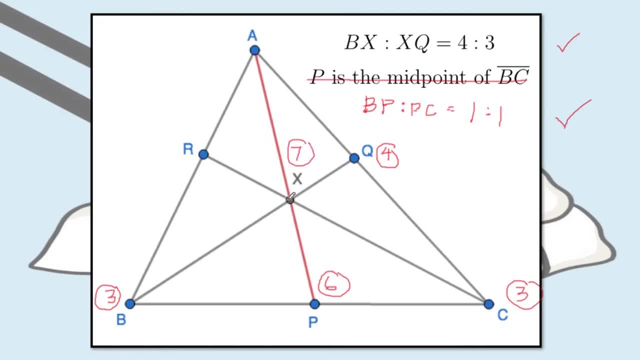 So the weight on X would be 7.. Now on segment AP. I know the weight on X is 7. So the weight of the weight on A should be 1, because 1 is the value that when added to 6, it gives a 7.. 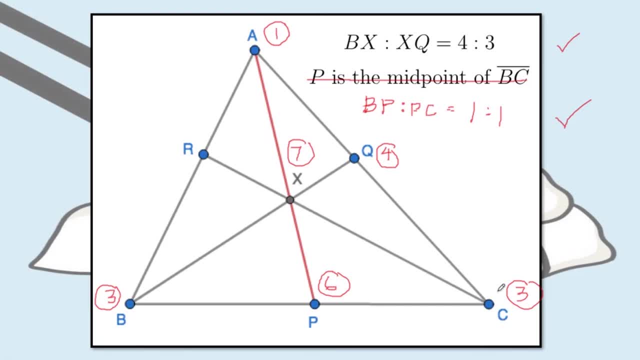 Now point R I can get via segment RC. So X is the point, X is the. the weight on X, 7 should be the sum of the weights on C and R And that gives me 4.. Or I can get 4 via, you know. 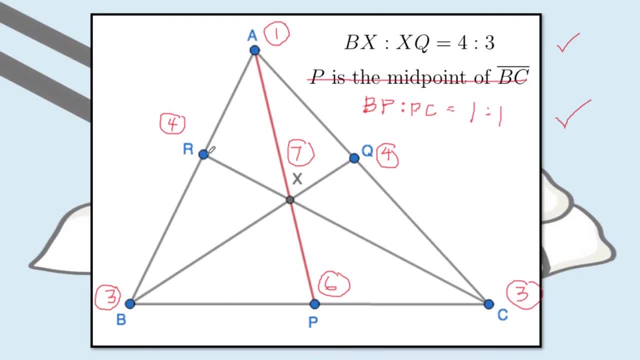 since segment A is 7.. So segment AB R is in segment AB. the weight on R would be simply A plus B or sorry, the mass of A plus the mass of B. So 1 plus 3, it gives you 4 either ways. 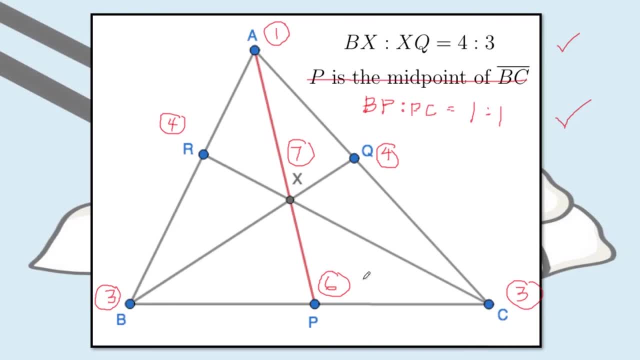 Now from here, let's just get a sample ratio that is not given. Suppose you want to get the ratio. AR is to RB, for example, AR over RB. Now, if you want to get AR over RB, you must get the mass of B over the mass of A. 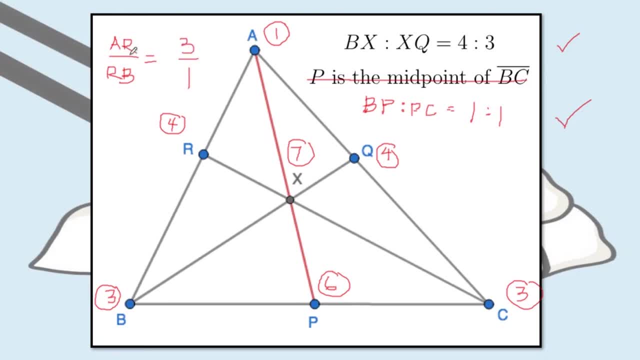 So the mass of B is 3 and the mass of A is 1.. So the ratio AR is to RB is actually 3 is to 1.. So this is how you do mass point geometry And hopefully you guys understood this video.